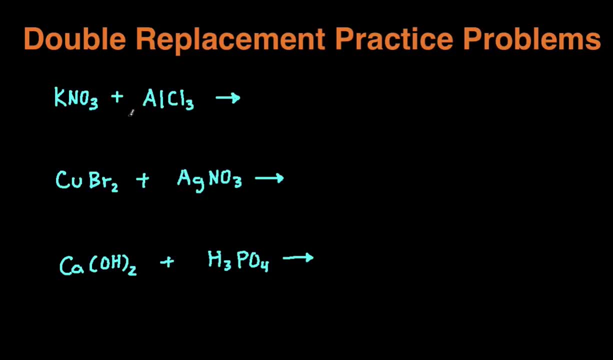 reacting with each other. the cations or the anions are going to switch places with each other. So what I mean by cations, they're positively charged and then anions are negatively charged. So essentially you can think of it as either the two positive charge ion switch places or the 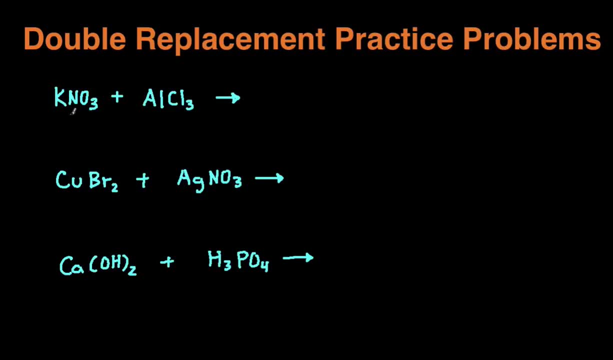 two negative ion switch places And it'll make a lot more sense as we go through these three practice problems together. So the first one is KnO3 plus AlCl3. So we're just going to predict the products. To do that, we first need to know what the charges of each of the ions are. 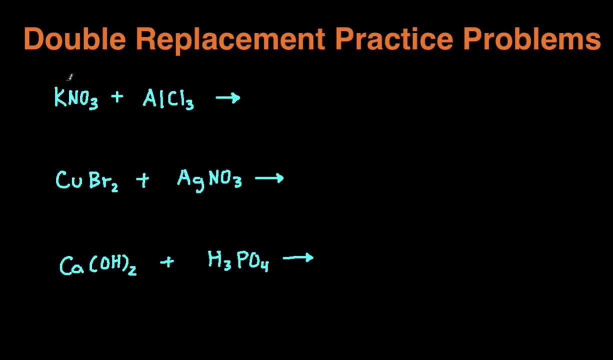 So in an ionic compound you're going to have a positive charge and a negative charge. So K, because it's in the first column of the periodic table- is going to be positive or negative One. and then nitrate is a polyatomic ion which has a charge of negative one. 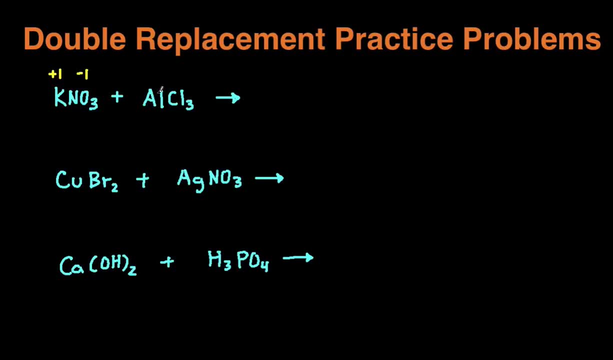 Then for aluminum chloride. aluminum is in the third main group of the periodic table, so it's going to have a charge of positive three, And then chlorine is going to have a charge of negative one because it's a halogen. Then what you do is you take your two positive charges. 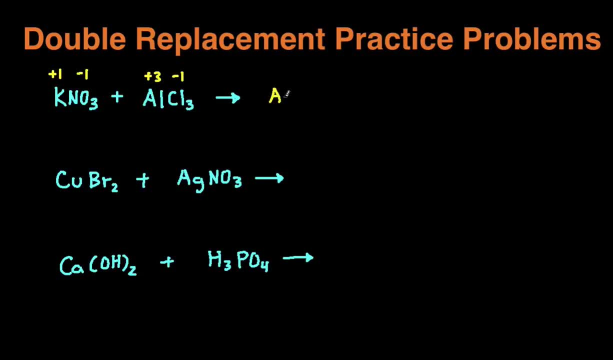 and then you switch places. So you get AlNO3 and then you get K- Cl. So two things I want you to pay attention here. First of all, notice the positive charge element always come first. So the Al came first and then K came first, because they'd 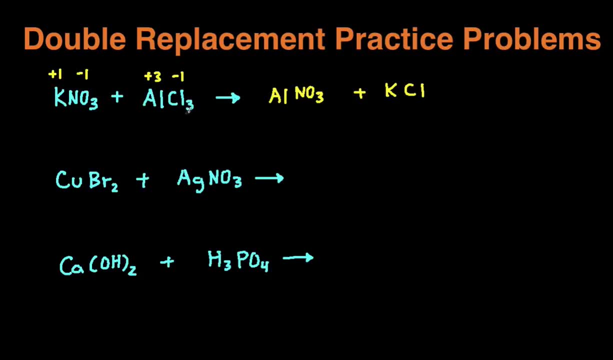 positively charged. Secondly, I want you to notice that, although there's three Cl's here, I only brought one over to the other side, And the reason why is because we want to make sure the charges are balanced. So what we're going to do is we're going to carry the charges over. Aluminum has a positive three charge And nitrate has a positive three charge, So we're just going to be carrying the two charges over all, over the three layers we're looking to illustrate. The nitrate has a positive three charge and the années has a positive three charge. 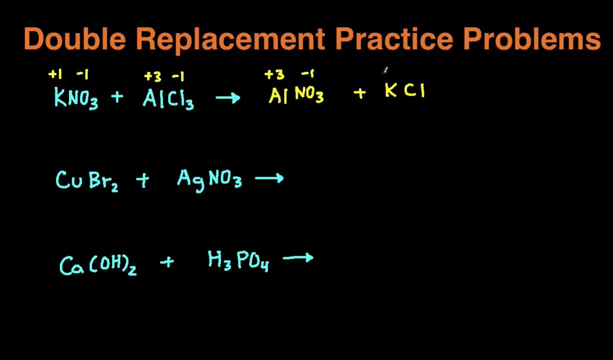 And so you can have a littleコnclusion when using the same product. When we're getting high blue bond soluble and aligned effects and all 3 Tamb Stick mixtures are coming together, charge and nitrate has a negative 1 charge, potassium has a positive 1 charge and chlorine. 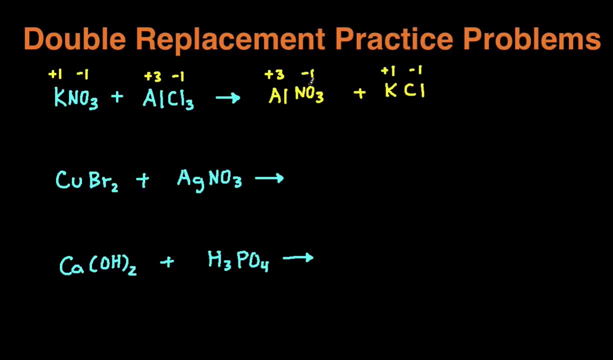 has a negative 1 charge. So now we check if the charges are neutralized, So aluminum's positive 3, nitrate's negative 1, that doesn't cancel out. So what we do is we can use the crisscross method so we can bring the 1 over and make 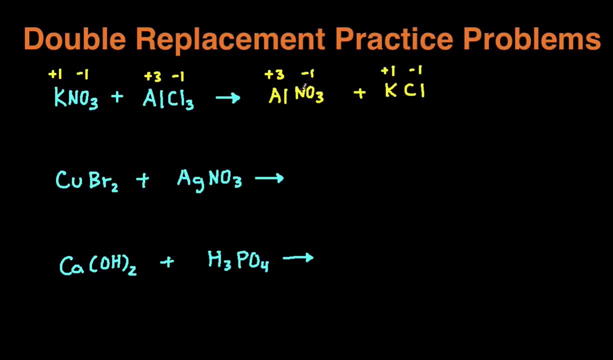 it the subscript of the aluminum, and then we can take the 3 and make it the subscript of the nitrate, And then on the KCl side you can see that both ions cancel out, because positive 1 and negative 1 cancel out and make it become neutral. 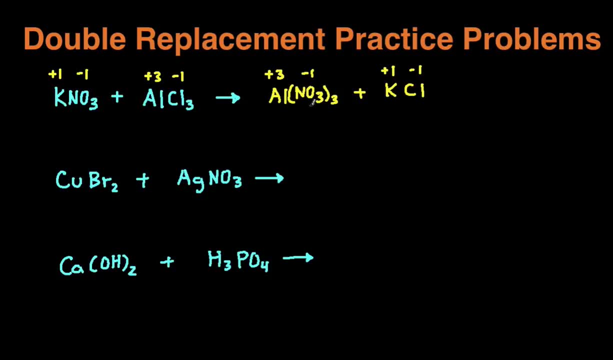 And then to complete this process, you would actually have to then balance the chemical equation and predict the states of the products. but I'm going to leave that for another video. This video I'm just going to teach you how to predict what the products are. 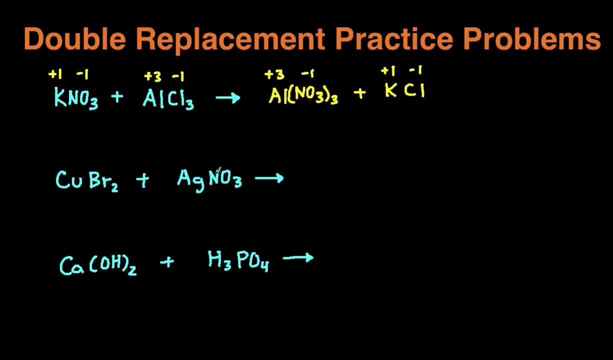 Then the next sample, copper bromide reacting with AgNO3,. so we're going to take the same step. first, We're going to determine the charge of each of the ions. Bromine is a halogen, so it's a negative 1 charge, and since we have two bromines, this 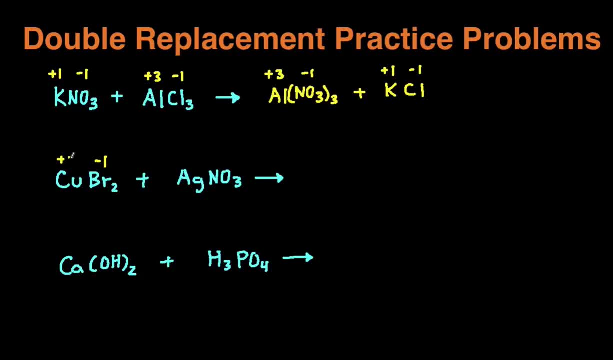 overall is negative 2, so copper then has to be positive 2.. And then Ag. although it's a transition metal, it always has a positive 1 charge, and nitrate again was a polyatomic ion with a negative 1 charge. 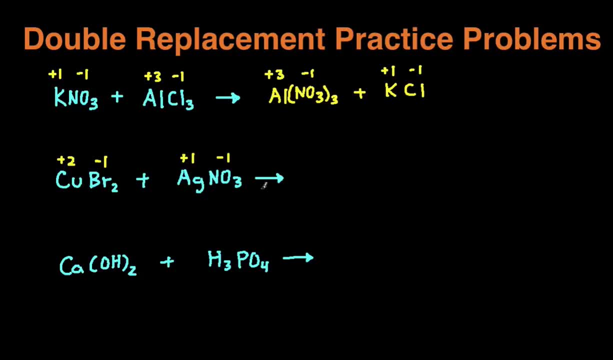 Then we're going to take our two positive ions, our cations, and switch places. So we get AgBr And I'm only taking one of each of the ions, I'm only taking one of each of the elements plus CuNO3, then carry the charges over. 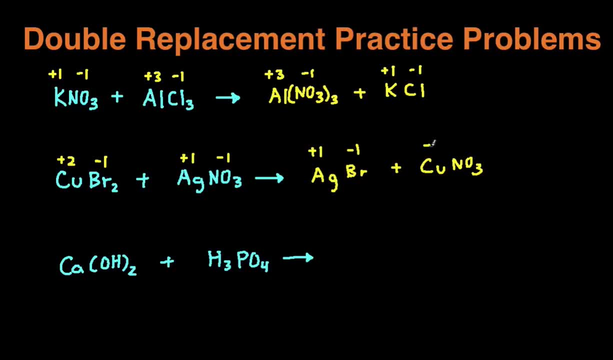 Ag is a positive 1 charge, bromine is a negative 1,, copper was a positive 2, and nitrate was negative 1.. Double check if the charges cancel each other out. Positive 1 and negative 1 cancel each other out. so this is just AgBr. 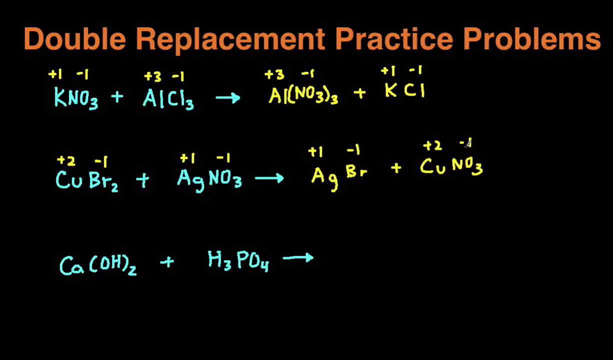 And positive 2 and negative 1 does not cancel each other out. so if they don't, then we use the criss-cross method. We bring the 1 over down here And then bring the 2 over down here, And then bring the 2 over here. 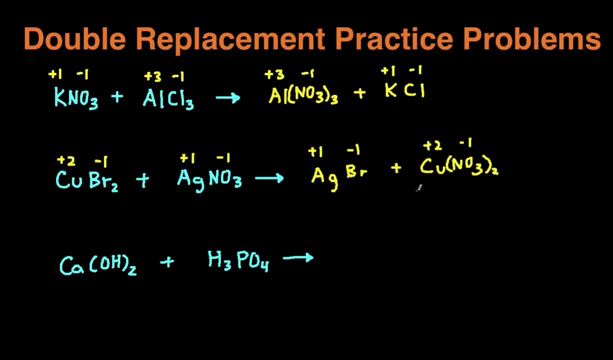 So we have 2 nitrates and 1 copper, And then the last example. so do the same steps over again. First step is just to write the charge. Calcium is in the second column of the periodic table, so it's going to have a positive 2. 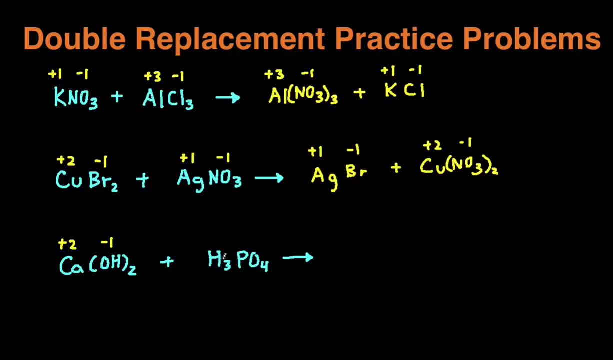 charge. Hydroxide is a polyatomic ion with a negative 1 charge. H right here is just positive 1 because it's in the first column of the periodic table. And then PO4 is a polyatomic ion with a negative 3 charge.